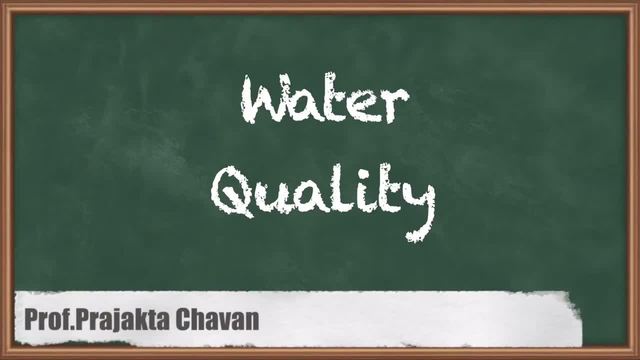 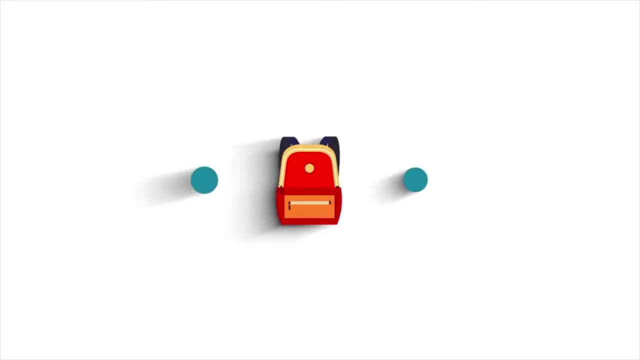 Hello everyone. In this lecture we are going to see water quality, or the characterization or characteristics of water, under the subject of environmental engineering work. As you all of know, water is how much important in our daily life, So water is an essential commodity to all life. Without water there can be no life. 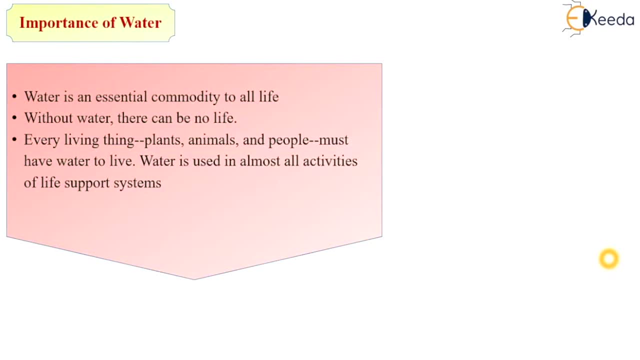 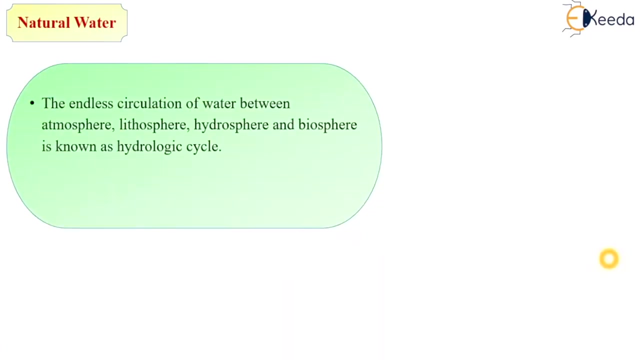 Every living things in form of plants, animals and people must have water to life. Water is used in almost all activities of life support system. Water is a major abiotic factor in the environment. Water is available in nature in different form, As we studied in school time. 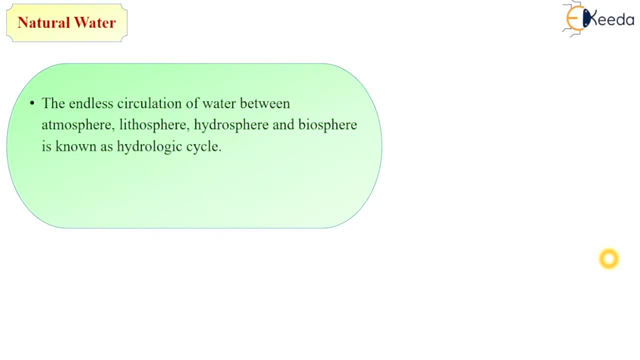 the hydrologic cycle. The endless circulation of water between atmosphere, lithosphere, hydrosphere and biosphere is known as hydrologic cycle, So we learnt this cycle many times. We get water from precipitation of water vapor in the atmosphere. Earth has tremendous amount of water. 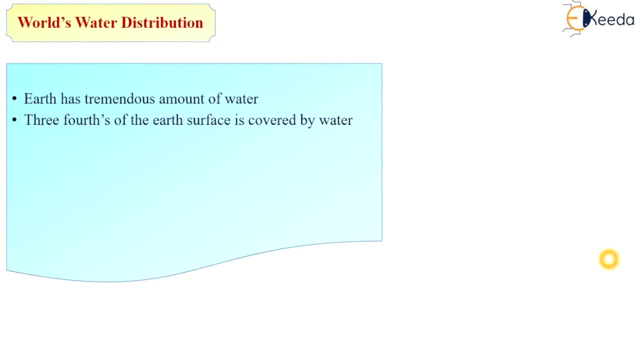 Almost 3 fourth of the earth's surface is offered by or covered by water, And 97% of world water is in the seas and oceans, So maximum amount of water is covered by seas and oceans. This water is saline water or it contains salt. 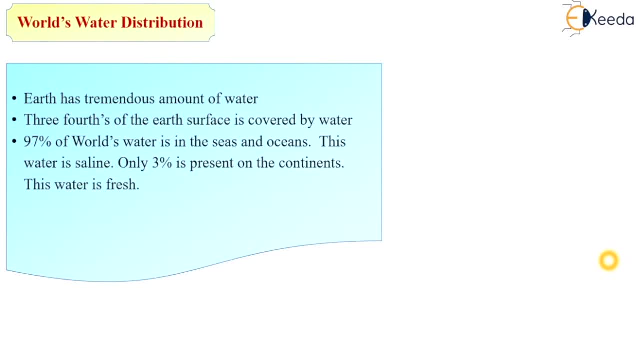 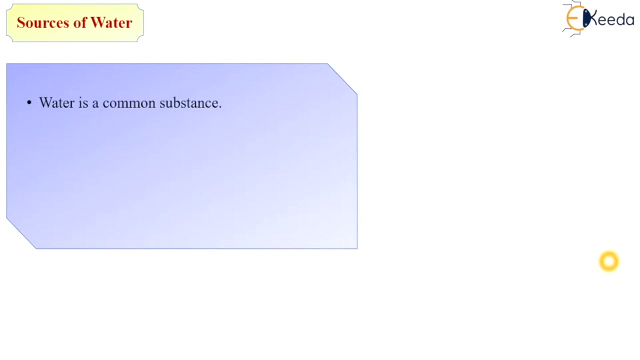 And only 3% is present on the continent. And this water is fresh in nature. So availability of fresh water is in very minor percentage. So the distribution of fresh water over land is uneven. So there are different sources of water. Water is common substance. 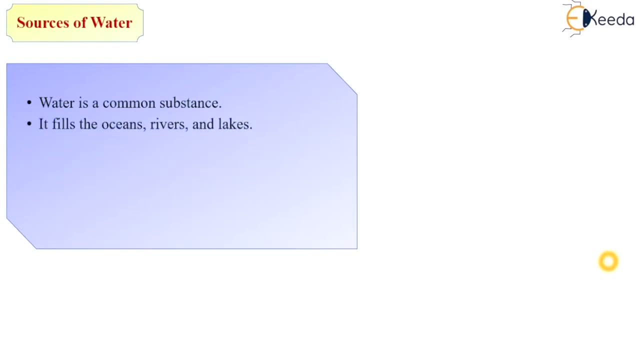 It fills the ocean, river and lakes, So, depending on its availability or capacity, it will be classified. It is in the ground and also in the air we breathe, So water is in everywhere. Water is used for drinking, all domestic purposes, agricultural purposes, industrial applications and cleaning and recreation. 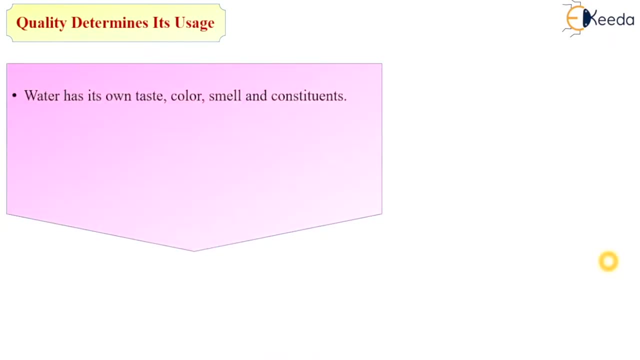 So to use the water in daily life, or for domestic use, or for agricultural use or for industrial activities, It is most important to know the quality of water And depending on its quality, we are apply this water for different purposes. Water has its own taste, color, smell and constituents. 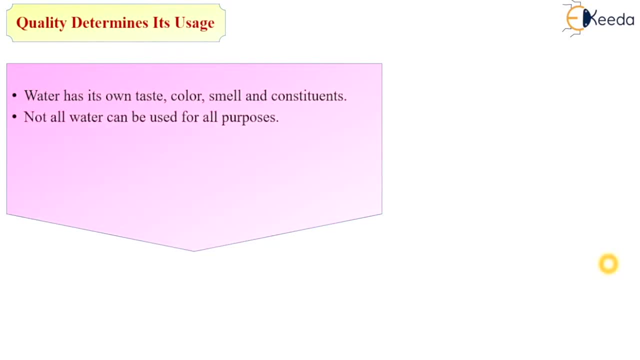 That is, contents. Not all water can be used for all purposes. For example, sea water cannot be used by us for drinking purpose. The suitability of water for different purposes is determined by its quality parameters. So what is quantity and quality of water? On an average, each person in a developed country use about 260 liter of water per day in the home. 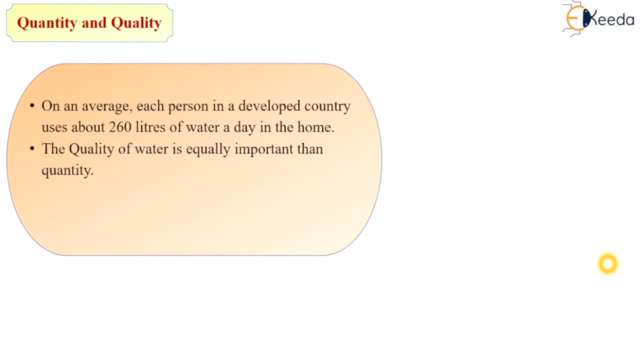 The quality of water is equally important than the quantity. Even if present in huge amount, we cannot use the salt water in many life support activities. So now what is? We are facing water scarcity problem, So for that, the recycling and reuse of water is necessary. 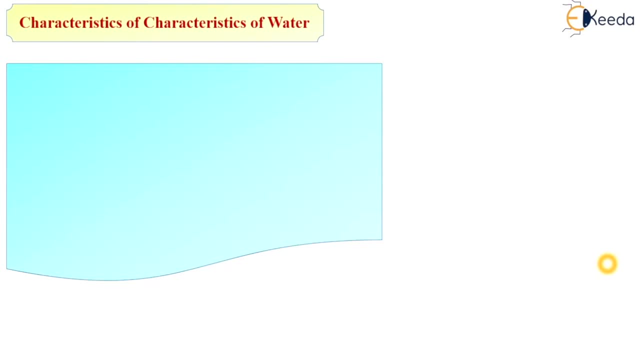 And for that to checking the quality of water is very important. So what are the characteristics of water? Water is a good solvent. Water never occur in its pure form. All water contains some amount of dissolved substances In form of impurities or in form of any biological parameters. 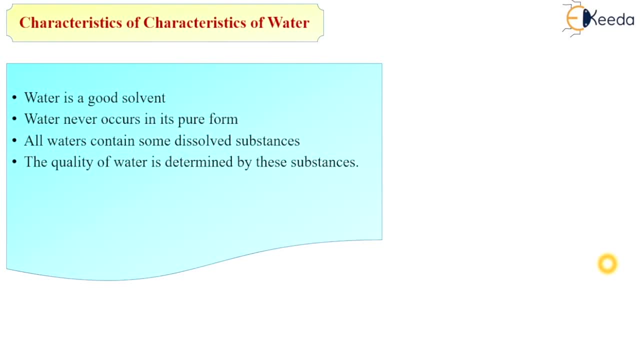 So the quality of water is determined by these substances. It has the ability to dissolve many inorganic and organic substances in water. So to know the characteristics of water, We will decide which treatment we are going to apply for this water. To treat the water and use it for drinking purpose. 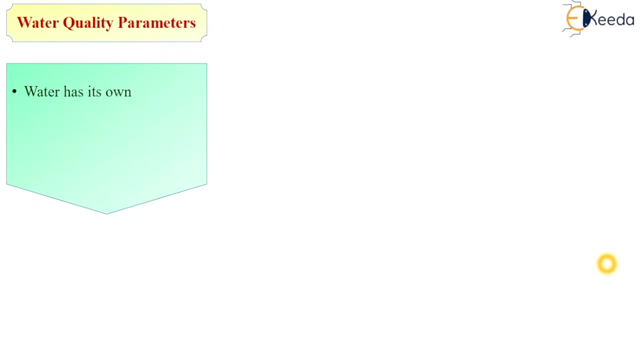 So there are different characteristics in form of physical, chemical and biological properties. So let's see one by one. So first is physical property. Under physical property We are classified the parameters as temperature, colour, odour, turbidity, electrical conductivity. 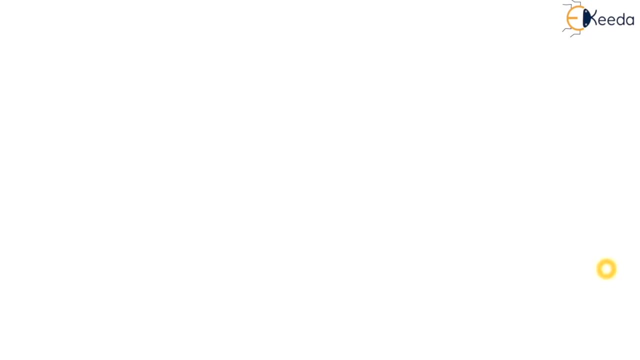 So these are the physical parameters. Let's see one by one parameter. So first, most important is temperature of water. It is essential for all environmental studies. It controls many ecological processes, Including chemical reactions, So chemical reactions occurring in lake, ocean or sea water. 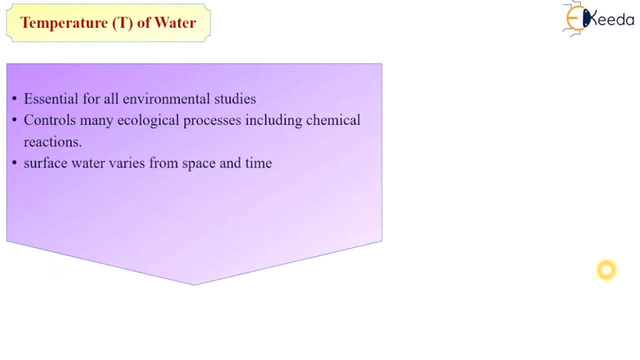 Which is depends on the temperature of water. Surface water varies from space and time. Ground water varies not only with reference to space and time, But also with reference to depth. So temperature is very much important, While characterisation of ground water, Because it is vary with reference to its depth. 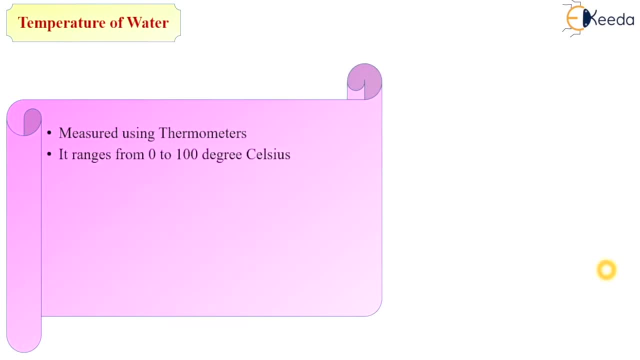 Temperature is measured using thermometer. It ranges from 0 to 100 degree Celsius. Unit of measurement is generally in degree Celsius. The temperature of surface water Is influenced by the atmospheric conditions. The temperature of ground water is controlled by The thermal characteristics of bedrock and depth. 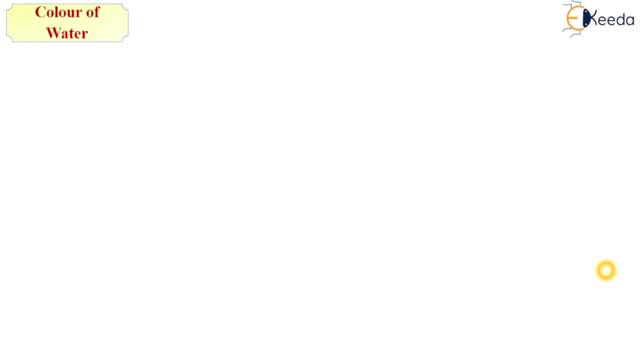 Next important physical parameter is colour of water. The colour of water is due to the suspended particles And organic matters present in water. ranges from light to dark brown. So colour import to the impact in the water Because of the suspended impurities present in water. 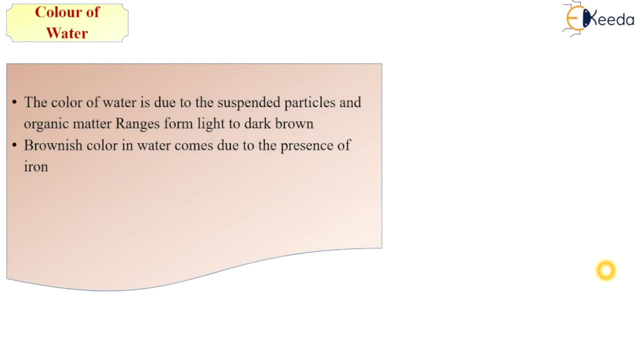 Brownish colour in water comes due to the presence of ions. Greenish colour in pond water is seen due to the presence of organic substances Including algae. Next physical parameter is odour. Pure water is odourless When water dissolves other substances. 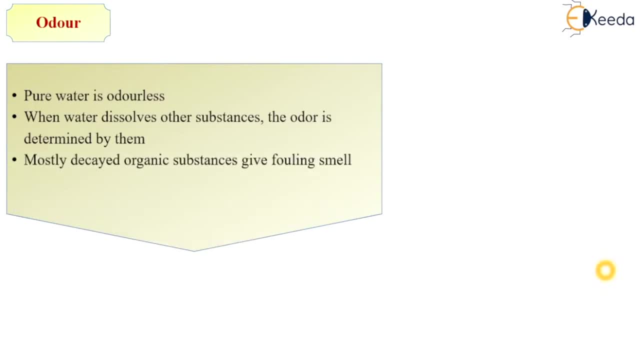 The odour is determined by them. Mostly decayed organic substances give fouling smell. Inorganic substances give earthy smell. So your drinking water should be free from odour Or it should be a odourless. Next important physical parameter is turbidity. 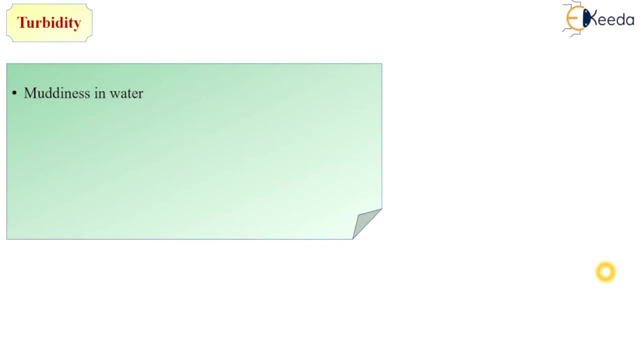 Turbidity is nothing but muddiness in water, And it is occur or present in water Because of it contains some suspended particles or impurities, Either in form of organic or inorganic in nature. So turbidity comes due to suspended particles from clay, silt and organic matter. 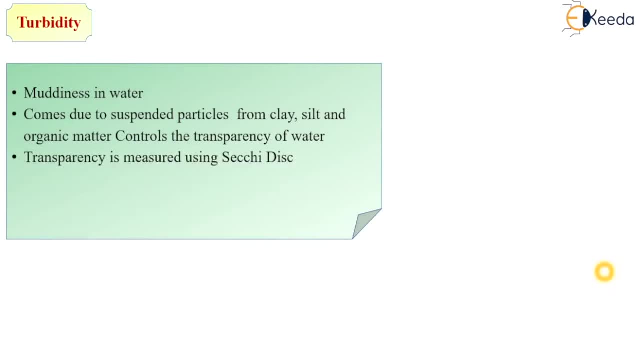 Controls the transparency of water. Transparency is measured using Satchi's disk. Water turbidity is measured using Nephthalometer. Next parameter is electrical conductivity. Electrical conductivity is The ability of substances to conduct an electrical current. The presence of charged ionic species makes water conductive. 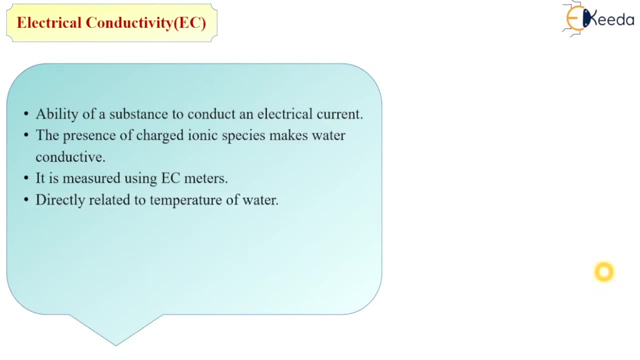 It is measured using electrical conductivity meter And it is directly related to temperature of water. Unit of measurement is Mohr's circles per centimetre at standard temperature And the range of the electrical conductivity values is 100 to 1 lakh. Next characteristic is: 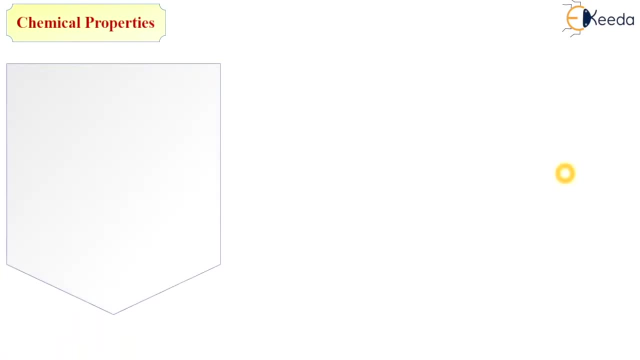 Chemical properties. So what are the parameters? comes under chemical properties. It includes pH, Total dissolved solids, that is, TDS, Major ions, Minor or trace elements, Hardness, Salinity And alkalinity. So let's we see one by one chemical parameter. 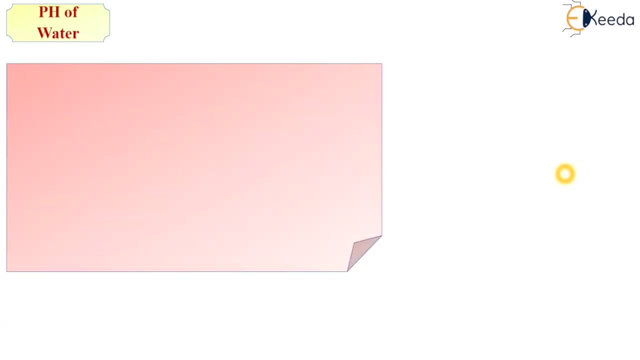 First is pH of water. To know the value of pH of water is very much important, So it should decide the water should be either in acidic or in alkaline nature, or it should be a neutral. It refers to the effective concentration of hydrogen ions in water. 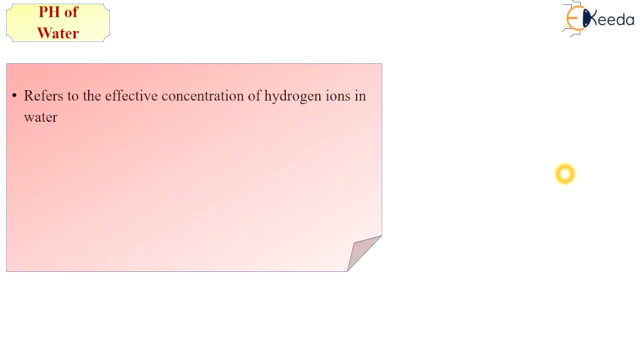 So pH scale or pH value, is representation of concentration of hydrogen ions present in water. It ranges from 0 to 14.. So the value of pH is ranges from 0 to 14.. Measured using pH meter, Water is said to be acidic if its value is less than 7.. 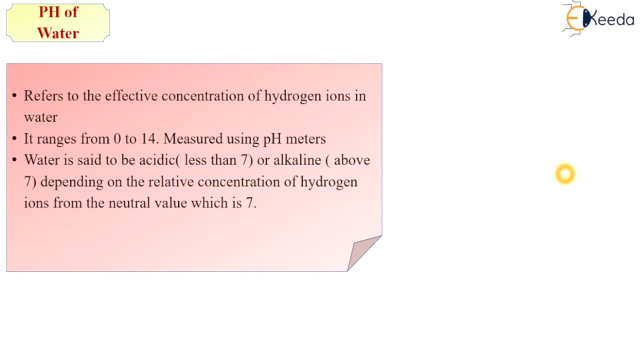 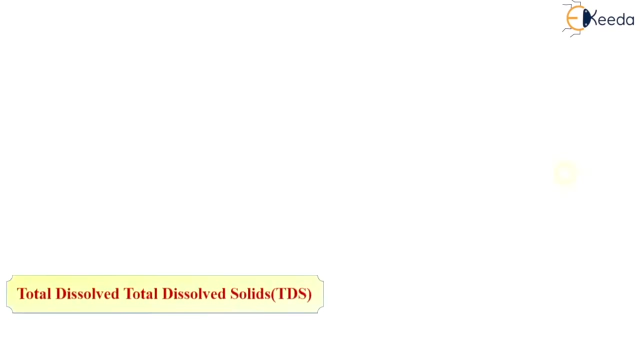 Or it refers alkaline when its value is above 7.. So less than 7 is acidic water and greater than 7 is alkaline water, Depending on the relative concentration of hydrogen ions from Neutral value, which is 7.. So if value of pH is 7, then that means the water is neutral. 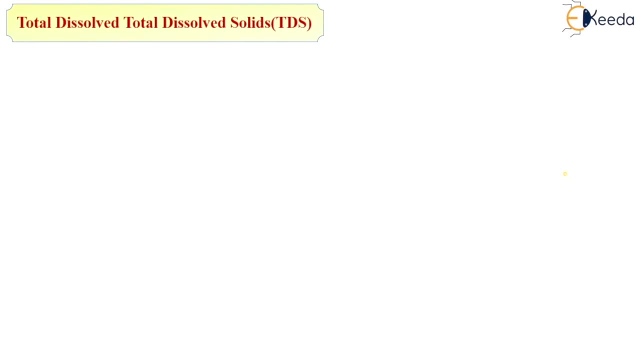 Next parameter is total dissolved solids: Concentration of non-volatile substances present in colloidal or molecular state And the measurement of this. Colloidal and molecular particles present in water That are nothing but the total dissolved solids in water, The total of all ions present in water expressed in part per million, that is, ppm or milligram per liter. 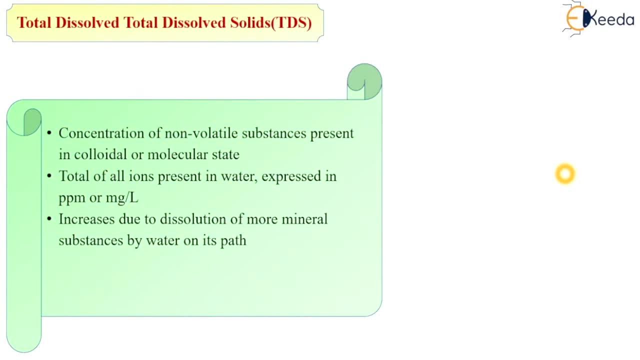 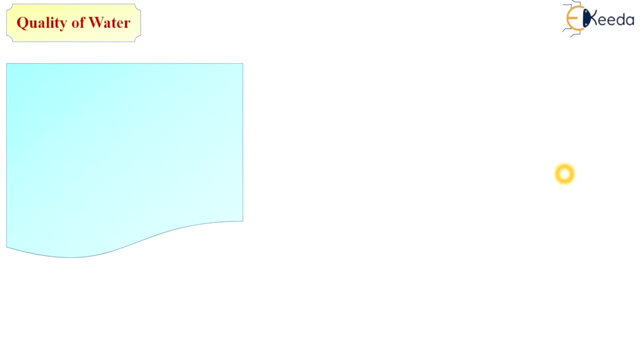 It increases due to dissolution of more mineral substances by water on its part. Total dissolved solids determine the suitability of water for all ions present in water, Different use and consumptions. So the quality of water is dependent on the total dissolved solids present in water. 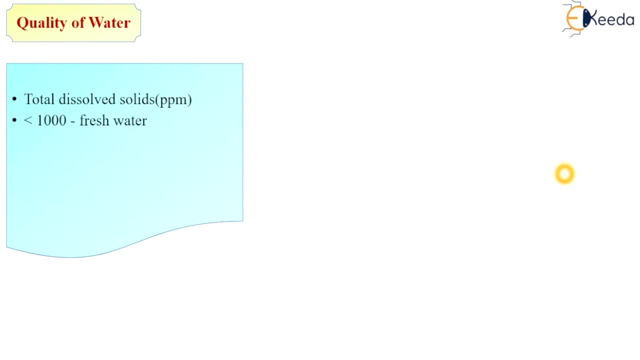 Total dissolved solids. for fresh water it should be less than 1000.. For brackish water, it should be in the range between 1000 to 10000.. For saline water, the quantity of total dissolved solids are in the range of 10000 to 1 lakh. 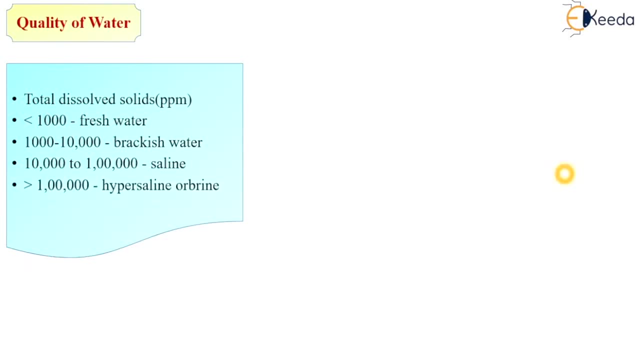 And for hypersaline carbine or particles the value should be greater than 1 lakh. So from these values we are classifying the type of water, whether it is fresh water, saline water, brackish water or hypersaline water. 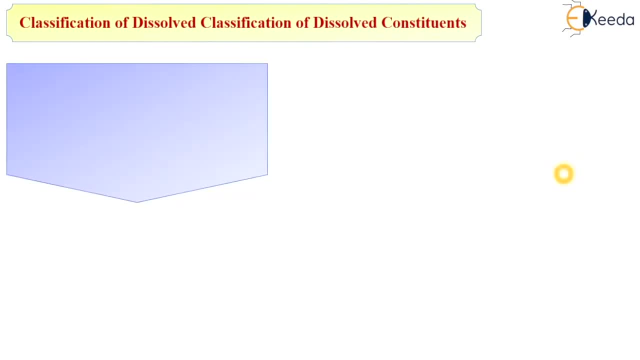 Classification of dissolved constituents. Basis of concentration in milligram per liter or charges, that is, positive or negative, or level of toxicity. So the dissolved constituents formation, or to know the quantity of dissolved constituents, is in form of either in milligram per liter, Or it should be varied from the charges, that is, whether it is positive or negative charge, or the level of toxicity. 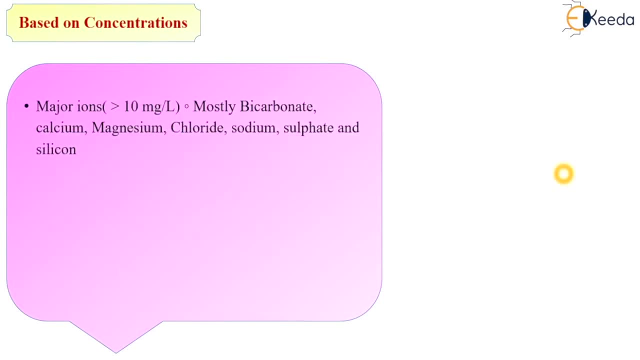 Based on concentration. the major ions should be greater than 10 mg per liter, mostly bicarbonates, calcium, magnesium, chloride, sodium, sulphate and silicon. Minor ions should be less than 10 mg per liter. Major ions are present in the range of 0.1 to 10 mg per liter. 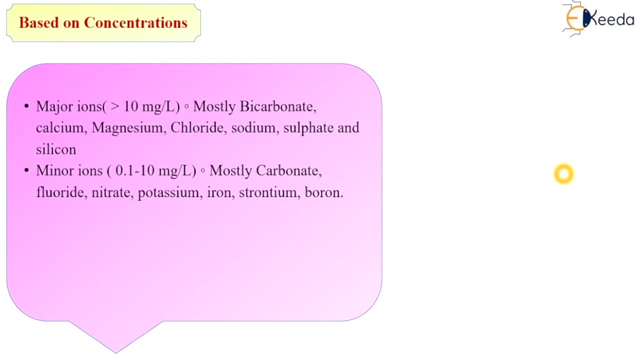 Mostly it includes carbonates, fluoride nitrate, potassium ion, strontium, boron, etc. And in water, trace elements sometimes are present which are in the range of less than 0.1 mg per liter In the form of aluminum, arsenic, terium, boramite, calcium. 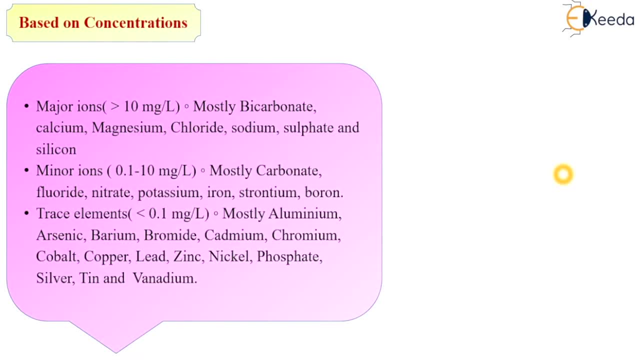 Poramide, Cadmium, Chromium, Cobalt, Copper, Lead, Zinc, Nickel, Phosphate, Silver, Tin and Vanipden. To know the quantity of trace elements in water are very much important Because if this quantity is exceeded, it should be a toxic or dangerous for the consumption. 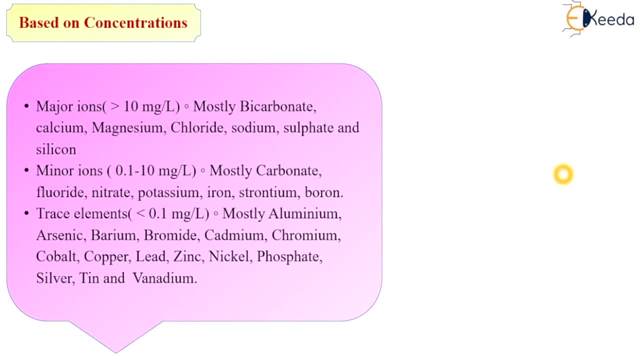 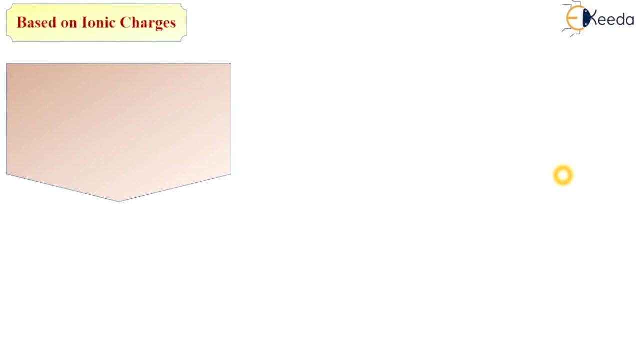 So the range present in its range present in water is very minor, but its effects are very harmful when its quantity range is exceeded. So we are find out the quantity of this trace element while we are analyzing the water characteristics. Based on ionic charges, it should be classified as major ion. 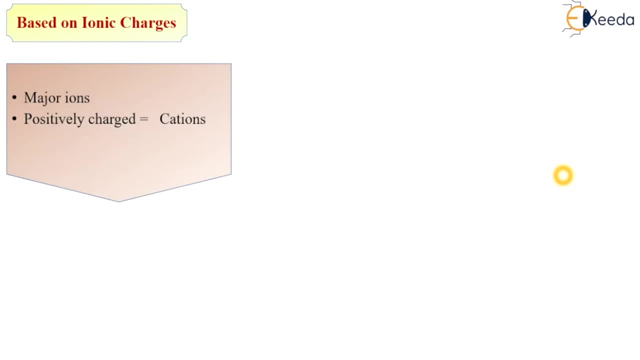 Major ions are the ions present in water, So positively charged ions- we are known as cations, and negatively charged particles, we are known as anions. So in water the particles are present in form of cations and anions. Major cations present in water are Calcium, Magnesium, Sodium, Potassium. 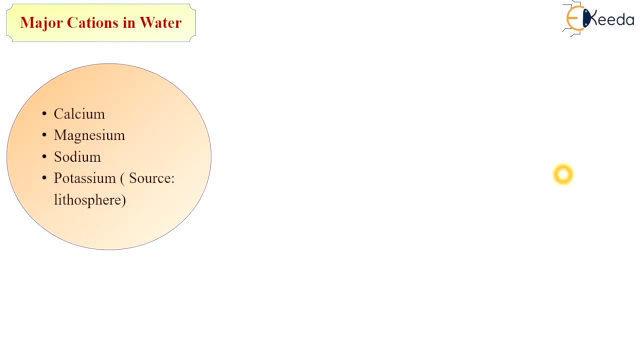 So in water, the particles are present in form of cations and anions. So in water, the particles are present in form of cations and anions. These cations, sometimes, which are required for the body while we are consuming fresh water. These cations, sometimes, which are required for the body while we are consuming fresh water. 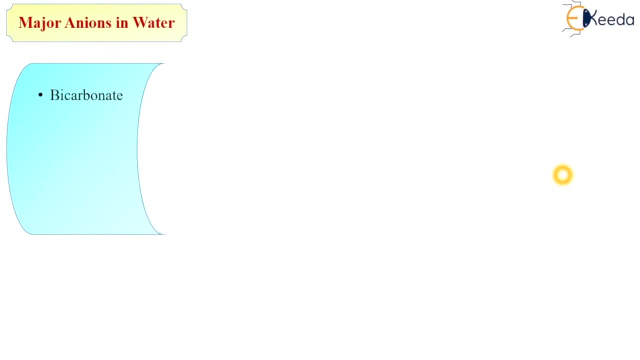 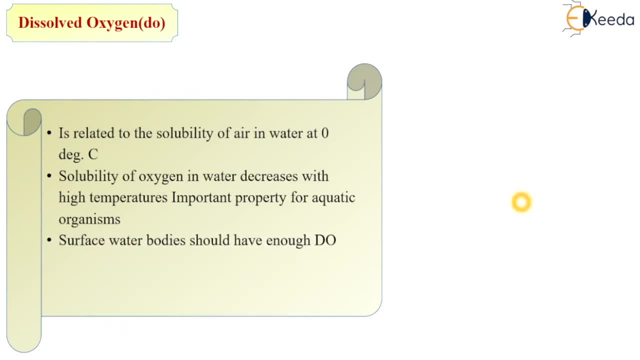 Major anions present in water is very minor, but again to know its quantity is very much important. factor: Major anions present in water is very minor, but again to know its quantity is very much important. factor: Surface water body should have have enough quantity of diesel oxygen. 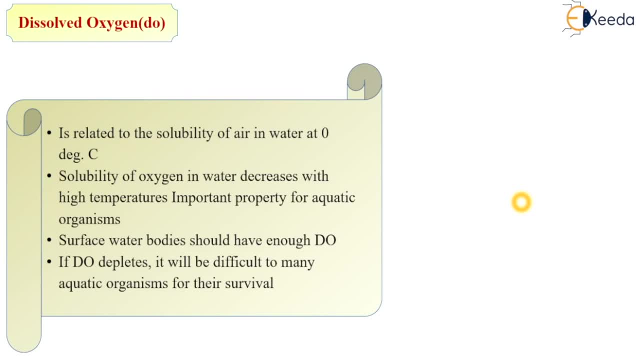 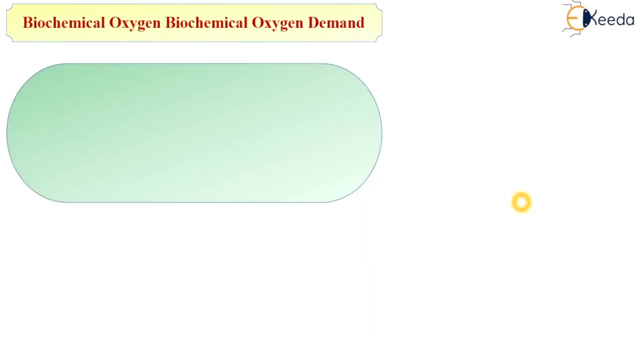 If DO depress, it will be difficult to many aquatic organism or their survivors. Next is Biochemical Oxygen Demand, or BOD. it is a major of biodegradable material. Next is Biochemical Oxygen Demand, or BOD. it is a major of biodegradable material. 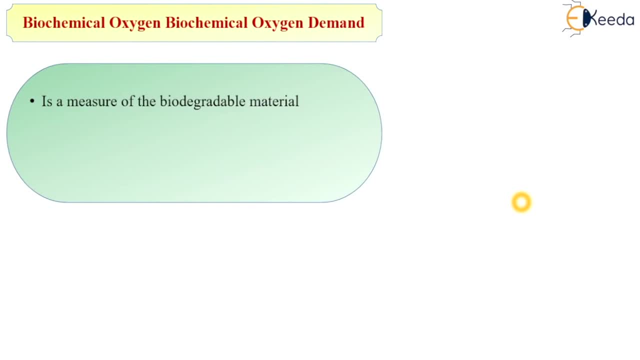 It is determine by intubating a water belly. It is determine by intubating a water belly. What would be part of this process. What would be part of this process? What would be part of this process? sample and measuring the decrease in dissolved oxygen as bacteria decomposes the material. 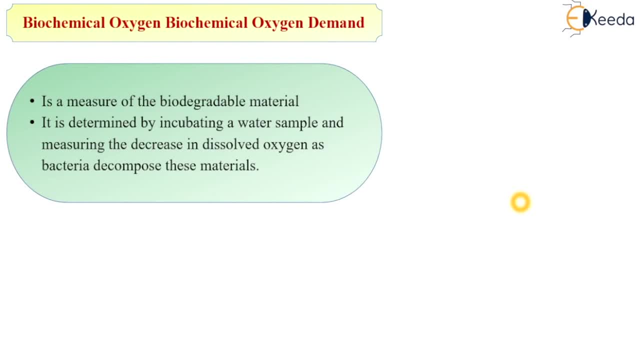 So biochemical oxygen demand is nothing but the organic matter, the oxygen required consume or to decompose the organic matter present in water, so that quantity is known as biochemical oxygen demand. that is nothing but the quantity of oxygen required for biochemically decomposition of organic matter present in water. in drinking water the value of BOD should be zero. that 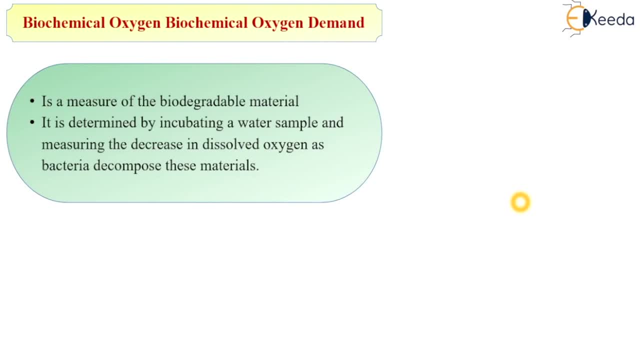 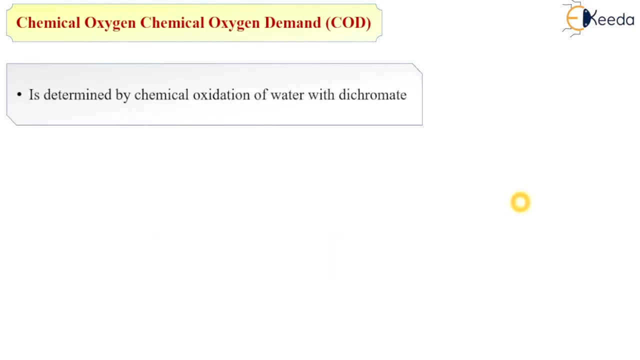 is the absence of biochemical oxygen demand, that is, absence of organic matters present in water. next is chemical oxygen demand. it determines chemical oxidation of water, which dipromete similar to BOD. the COD value for drinking water is also zero, so only dissolved oxygen is present in fresh water and other biological 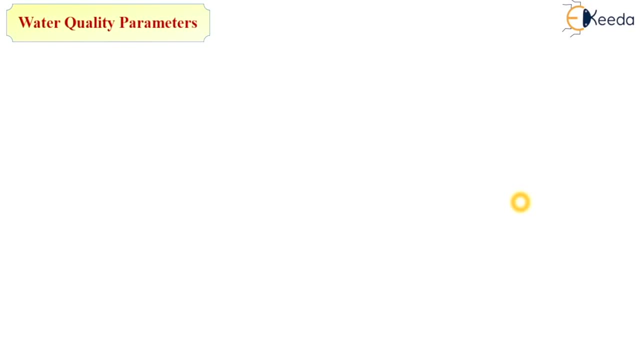 parameters are absent. so water quality parameters, the limits, its limits, the solubility of water for drinking water For different purposes, for drinking purpose, for domestic purpose, for agricultural purpose, for industrial purpose and for cleaning and recreation. and there are permissible limits for discharge standard of treated water. so there are different standards, methods are 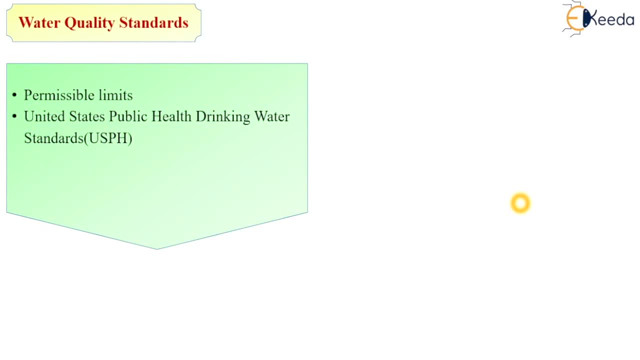 we are used for selecting the permissible limits. So sometimes we are referring United States public health drinking water standards, that is, USPA standards. sometimes we are referring Indian standards institutes, which is based on Indian conditions and worldwide parameters which we are going to use in form of World 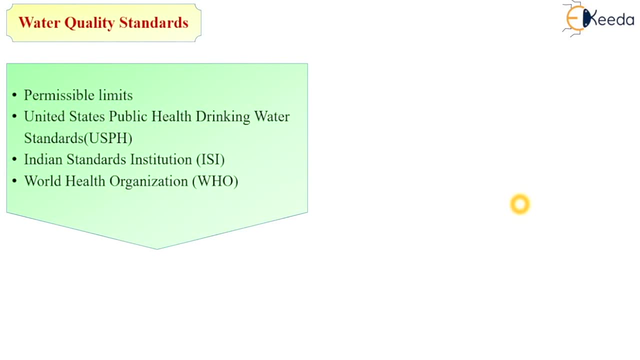 Health Organization standards, that is, WHO standards. So any one of ISI or WHO standards is used to determine the permissible limits of drinking water. So these are the home standards we are using while comparing the fresh water to the untreated or waste water. so these parameters we are going to see in next lecture. 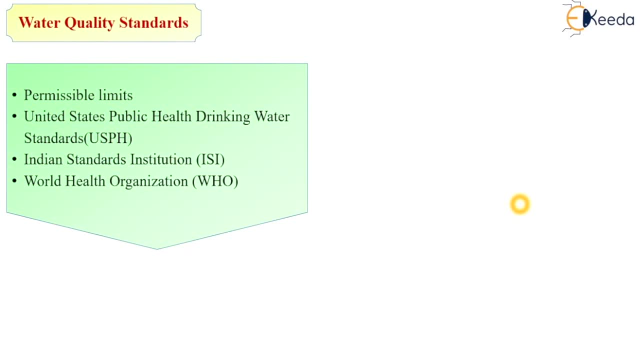 So the summary of this topic, or in this lecture, we have covering the following points, that is, the importance of water, The characteristics of water. The characteristics of water in form of physical, chemical and biological parameters or characteristics In physical parameters includes pH, turbidity, temperature, electrical conductivity, colour.